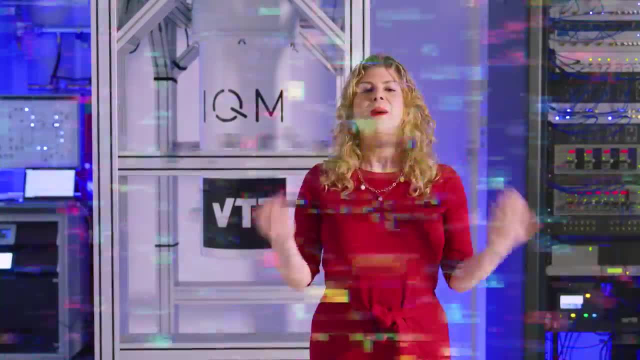 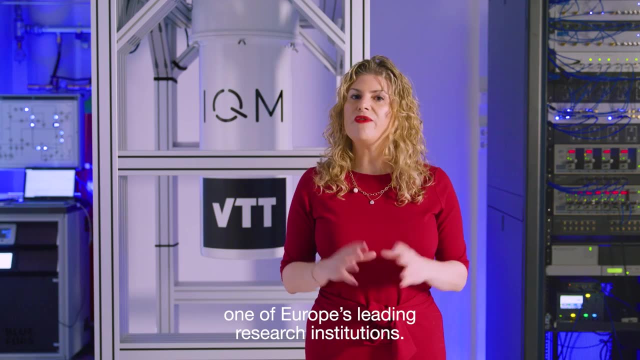 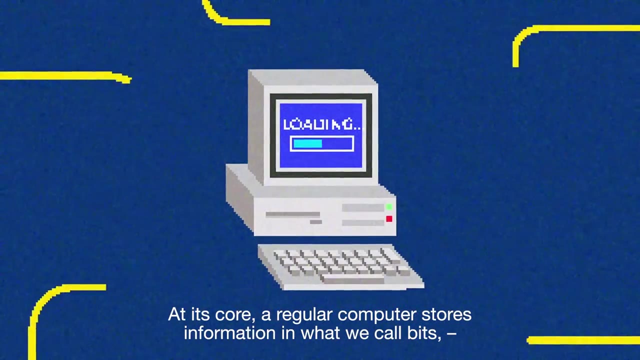 My name is Deborah Berebiches and I am a lead scientist in quantum computing at VTT, one of Europe's leading research institutions. Welcome to our video series: The Quantum Advantage. At its core, a regular computer stores information in what we call bits. 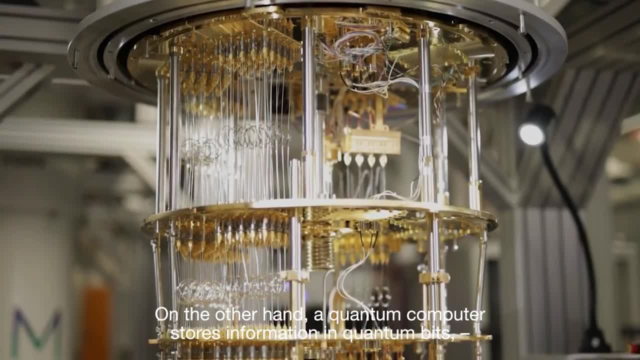 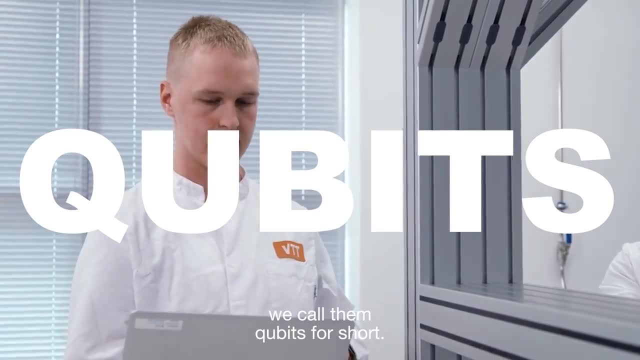 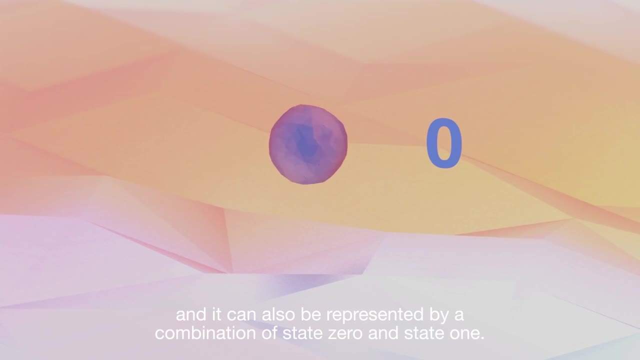 which are series of ones and zeros. On the other hand, a quantum computer stores information in quantum bits. We call them qubits for short. A qubit can be represented by a one or a zero, just like a classical bit, And it can also be represented by a combination of state, zero and 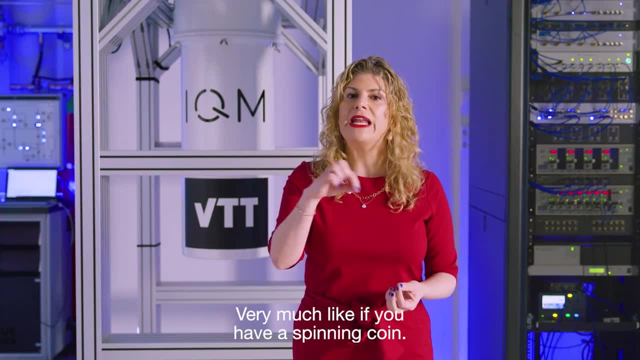 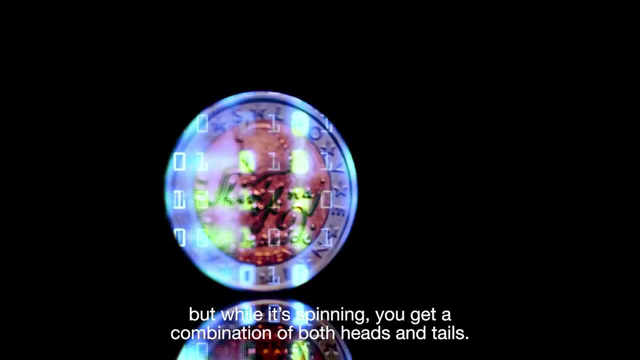 state one Very much like: if you have a spinning coin, you have two sides- heads and tails- but while it's spinning you get a combination of both heads and tails. The qubit is what makes a quantum computer unique In classical computer. 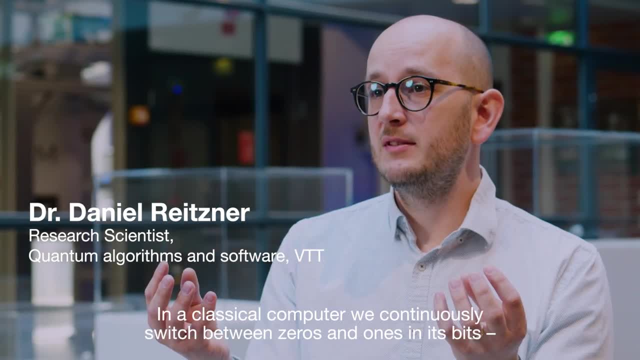 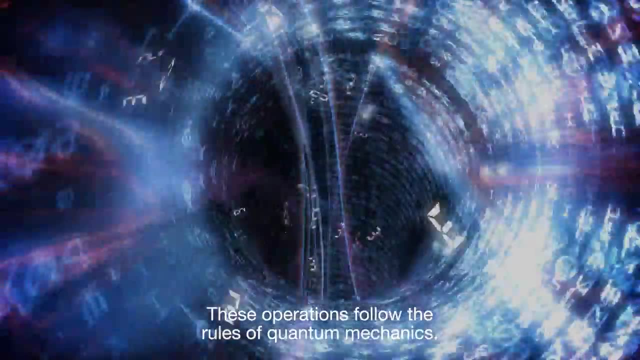 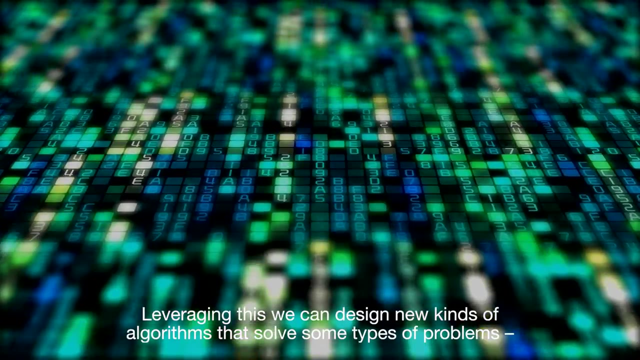 we continuously switch between zeros and ones in its bits to perform classical computations. But qubit is much more. We can perform more complex operations on it. These operations follow the rules of quantum mechanics And leveraging this we can design new kinds of algorithms that solve some types of problems much faster than the classical computers. Because a 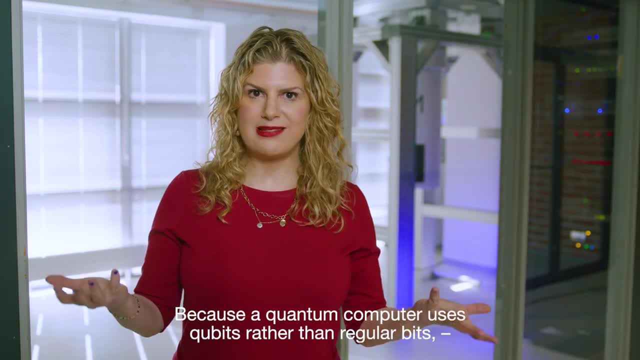 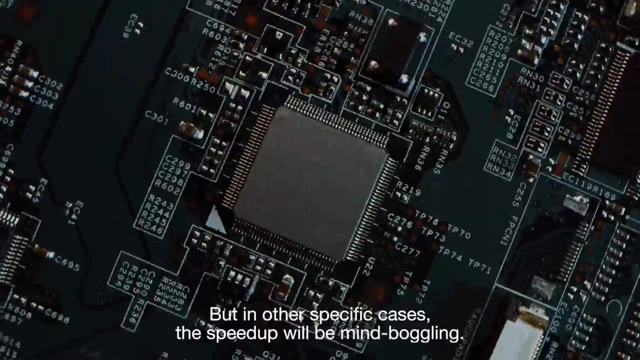 quantum computer uses qubits rather than regular bits, it can actually speed up some calculations. In some cases it can even hooked a bar ambulator to do computer justice on it. This means that a the speed-up would be modest, But in other specific cases the speed-up would. 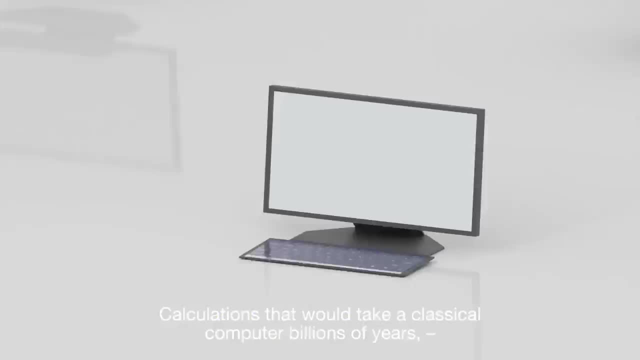 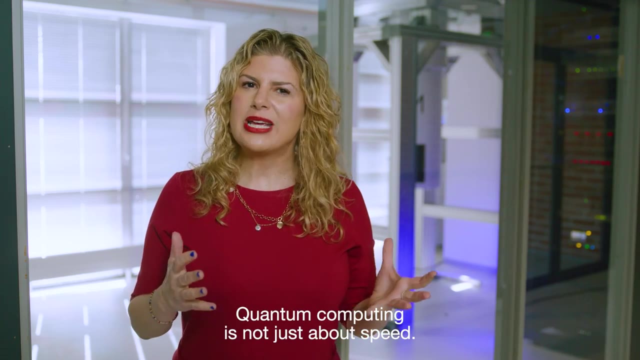 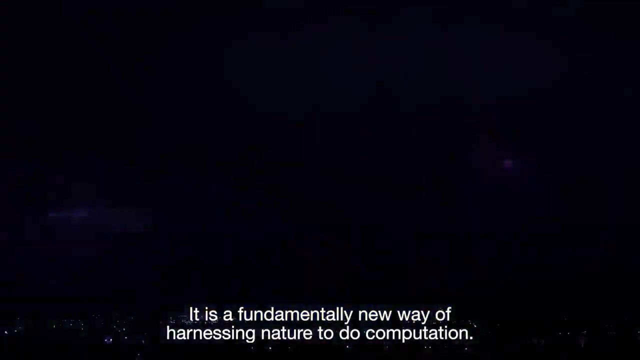 be mind-boggling. Calculations that would take a classical computer billions of years could be calculated with a quantum computer in the blink of an eye. Quantum computing is not just about speed. It's a fundamentally new way of harnessing nature to do computation, And that is why quantum computers can help. 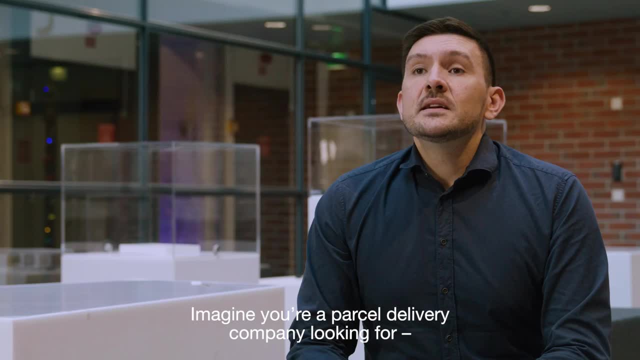 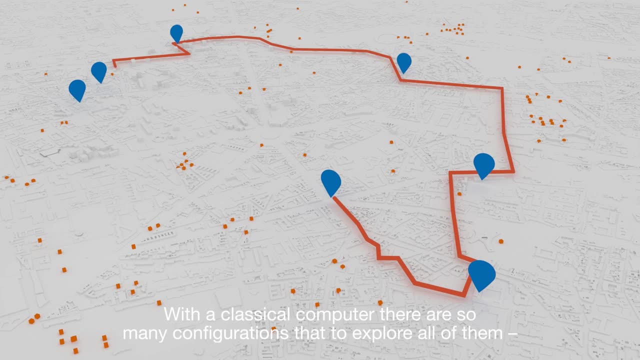 us tackle the really challenging problems on our wish list. Imagine you are a parcel delivery company looking for the fastest and cheapest way to deliver parcels to your customers. With a classical computer, there are so many configurations that to explore all of them it will take too.